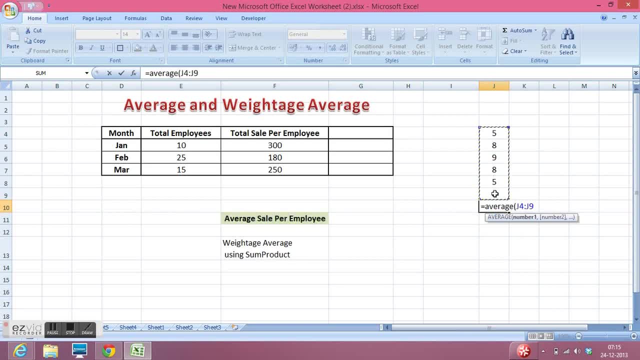 open parenthesis, We can select the data and close parenthesis. So average of this data set is 7.167.. Now if we have more than one variable and then we want to calculate average, so for doing that we need to calculate weightage average. Let me explain weightage average with. 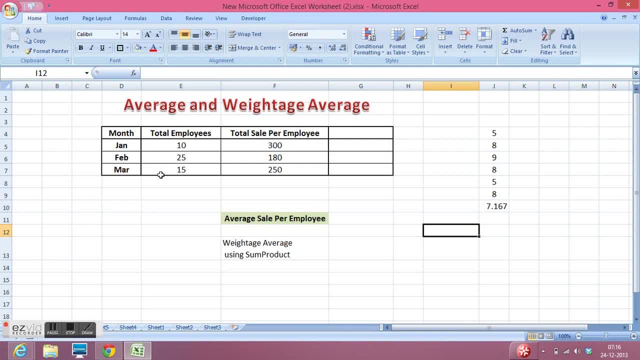 the help of one example. I have some data here where I have total employees and total sales per employee. In the month of Jan, 10 employees have given 300 sales per employee. So in the month of Jan total sales would be equal to 300 multiplied by 10.. In the same way we can: 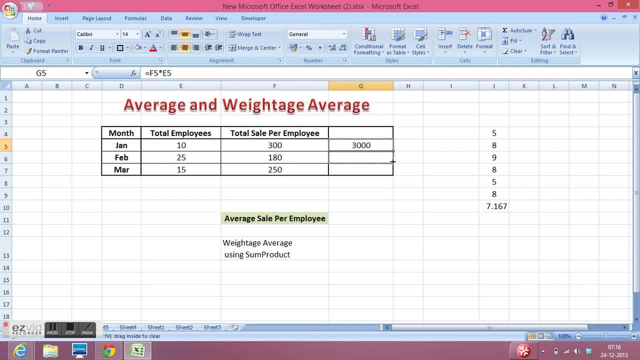 calculate the total sales per month for Feb and March. Let me write: Now I want to calculate average sales per employee. Now I want to calculate average sale per employee. For that we need to calculate weightage average. So how can we calculate that? I will take the sum of these three values equal to sum. 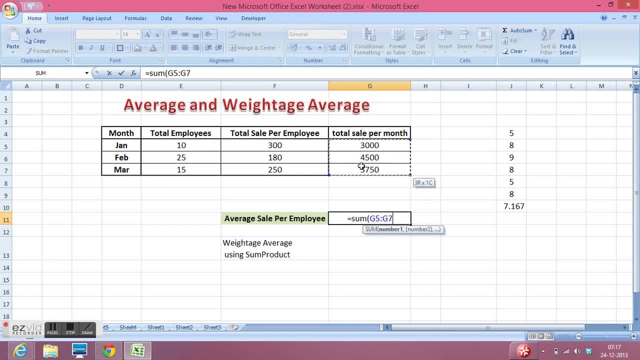 I will select these three values, Closed parenthesis, Divided by sum, I will select the total employees, Closed parenthesis Enter. So average sale per employee from this data is 200.. 225.. There is another way of calculating weightage average: using sum product formula. So how can we calculate weightage average using sum product? Let me write equal to sum product, Open parenthesis. 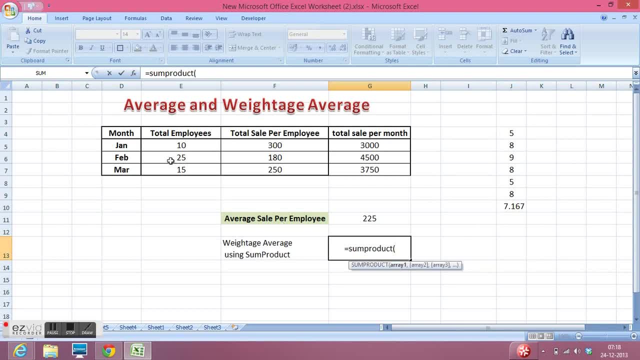 Then I need to select total employee Comma, Total sale per employee, Closed parenthesis, Divided by sum- Open parenthesis, Then total employees- Closed parenthesis, and Enter. So this is how we can calculate weightage average in one step, using sum, product and sum. 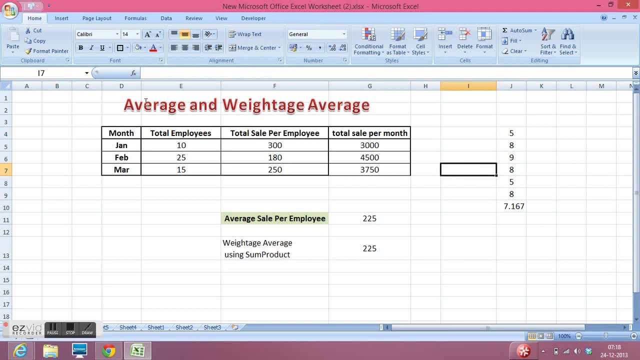 So this is how we can calculate average and weightage average in MS Excel. Thank you for watching watching this video. if you like my video, please subscribe to my channel. thank you. 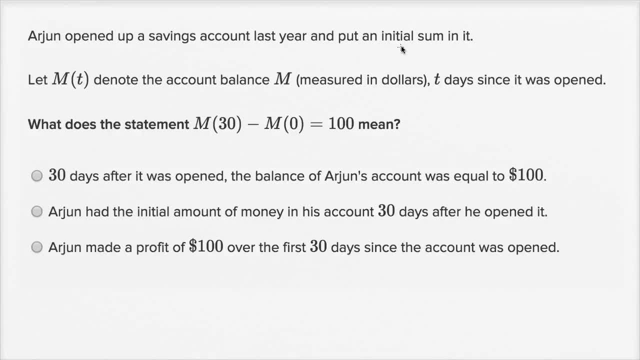 Arjun opened up a savings account last year and put an initial sum in it. Let m of t denote the account balance m measured in dollars t days since it was opened. What does the statement m of 30 minus m of zero, equaling 100 mean? 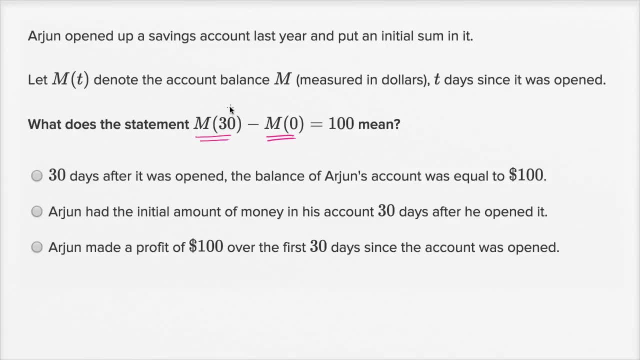 So, before I even look at the choices, let's think about it. This means when you input t equals 30 into your function, you're going to get m of 30. So let me make that clear. So if you say t is equal to 30,, 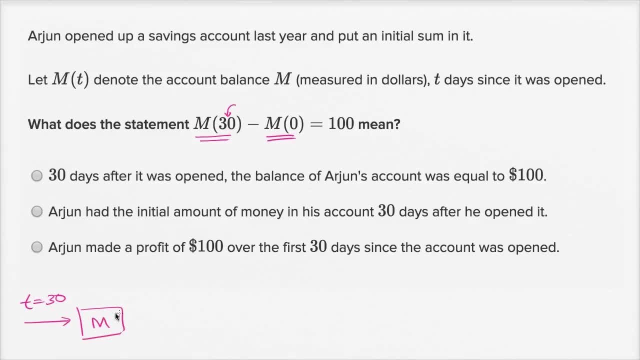 you input that into your function m, you are going to get m of 30. So one way to think about it is: this is the account balance 30 days since it was opened. This is when t is equal to 30.. This is the account balance after 30 days. 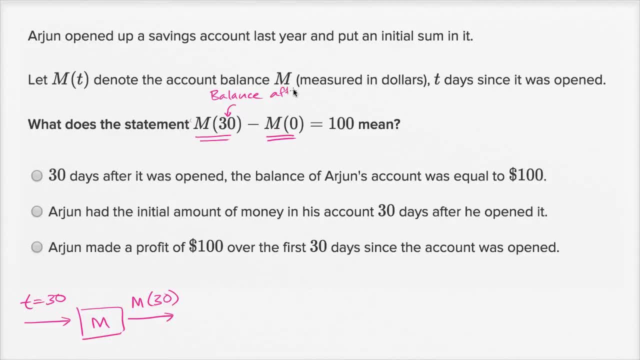 So let me write that down: Balance after 30 days. Now, by the same logic, this right over here: this is when we put t. when we set, t equals zero. This is the balance after zero days. Or you could say this is the initial balance. 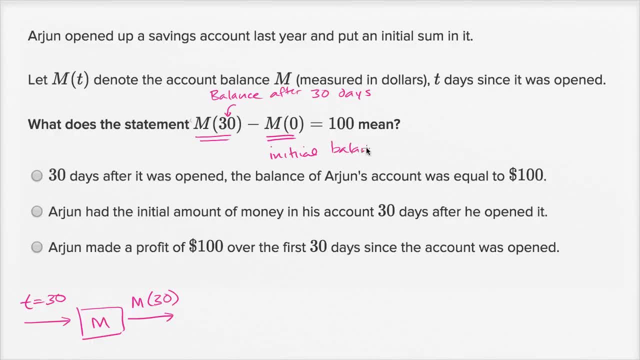 Initial initial balance. So what they're doing they're taking our balance after 30 days and from that they're subtracting the initial balance and they're saying that that's equal to 100.. So there's a couple of ways you could interpret this. 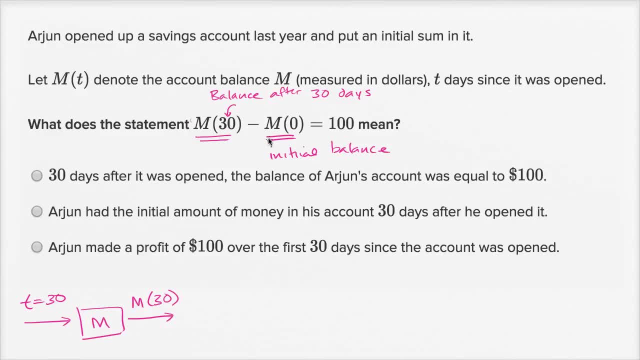 and I haven't even looked at these choices yet. We'll see if any of these match up. You could say that your balance after 30 days is 100.. You could say that your balance after 30 days is 100.. You could say that your balance after 30 days is 100.